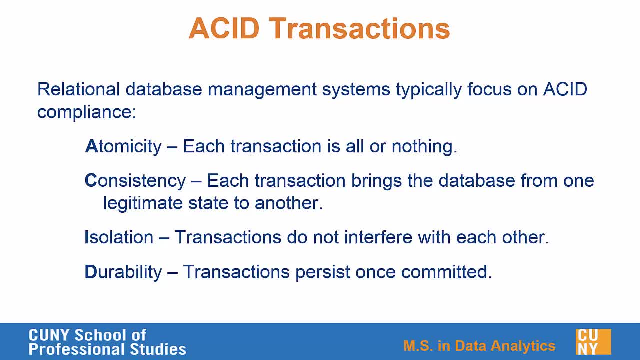 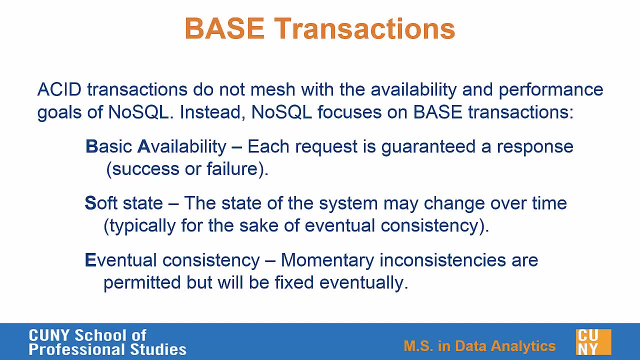 And it focuses on durability, Where, once a transaction occurs, it persists. Those are traditional focus points for relational databases. Sometimes we're more interested in performance, though, So a NoSQL solution is going to focus on availability and performance goals rather than ACID transactions. 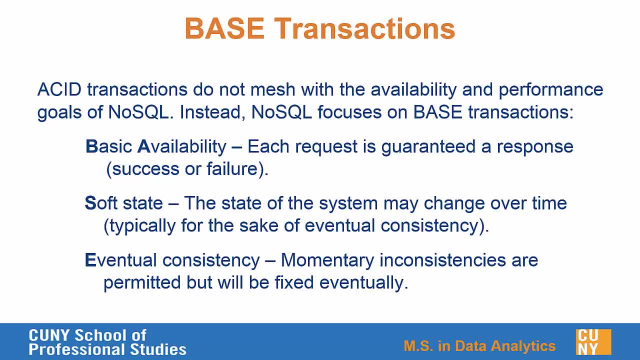 So basic availability is our primary goal. We want every request made of the database to be guaranteed a response of some sort. We want the database to be in a soft state, By which we mean it'll typically eventually reach consistency, but it may change over time as it moves toward consistency. 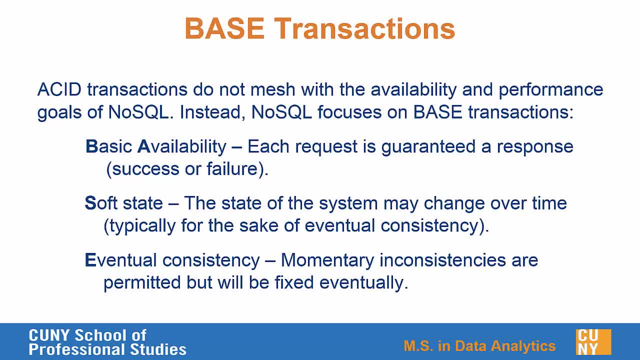 So at every given moment it's not in a consistent state. For example, if you have $1,000 in your bank account and you give me $1,000, a traditional relational database is going to want that $1,000 only to be in one place or the other at any given moment. 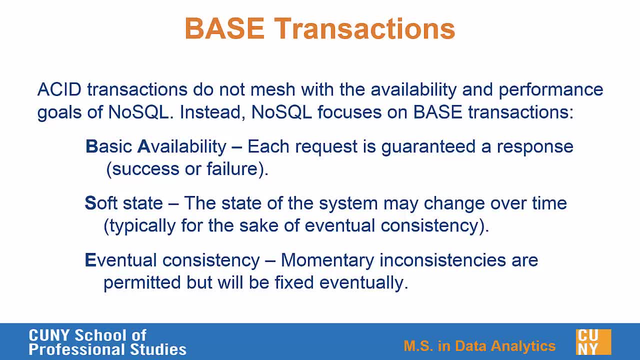 But in a soft state system, it's possible that the $1,000 will still be in your account while it also shows up in my account, So you'll have inconsistency there. right, We don't really have $2,000 there. 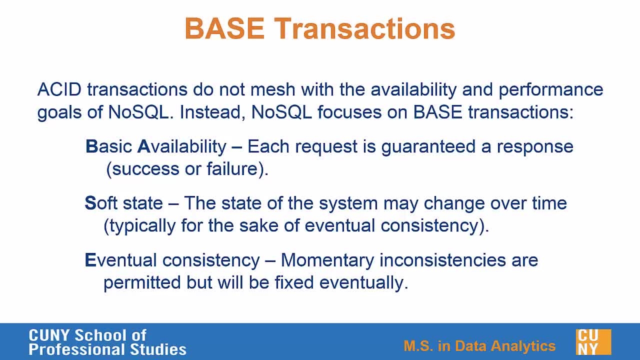 We just have it showing up in two different places. However, base transactions are eventually going to reach a state of consistency, So eventually that $1,000 will only show up in one account, But it might take a little bit of time And most of the time that momentary inconsistency really is for quite a small period. 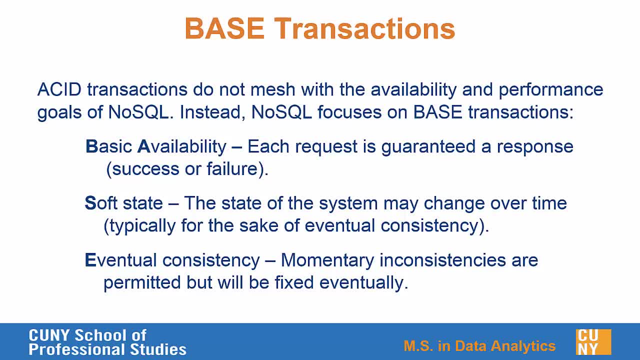 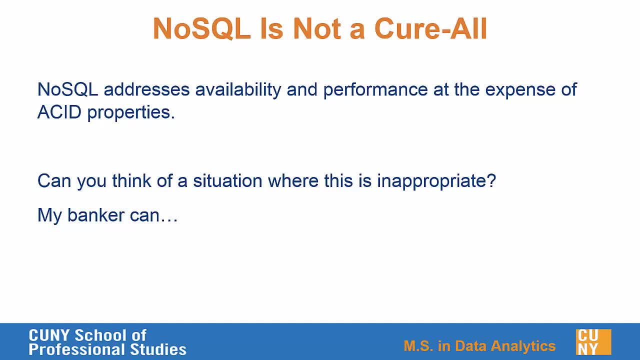 But it can persist for a long time, For a little bit of time. NoSQL is not a cure-all. It does give availability and performance advantages, but it does so at the expense of those asset properties. So keep in mind that example of the $1,000.. 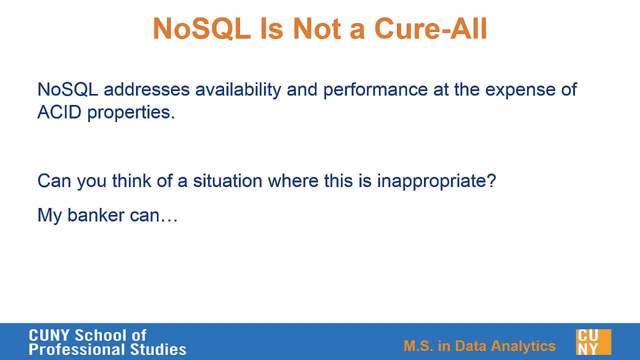 A banker would not be okay with that right. A banker is going to say that $1,000 has to be in either one account or the other. That transaction, once it occurs, it occurs And the money is only in one account. 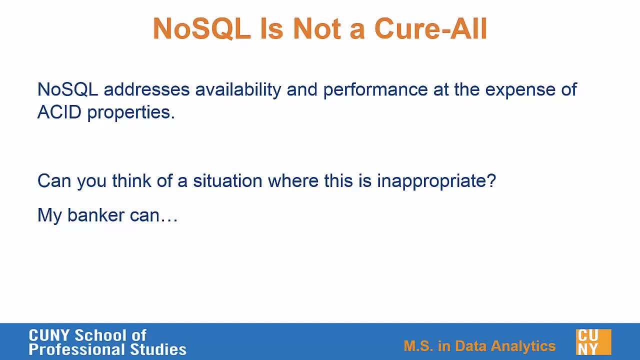 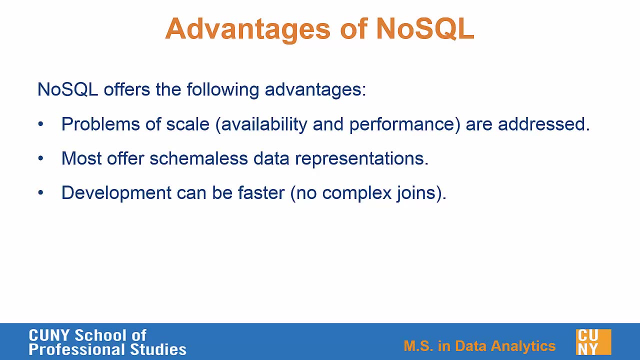 So NoSQL does have some disadvantages, If that transactional structure is very important. So keep in mind, when you might want to prefer a SQL solution and when you might want to prefer a NoSQL solution, Again, the advantages of NoSQL: It offers availability and performance advantages.